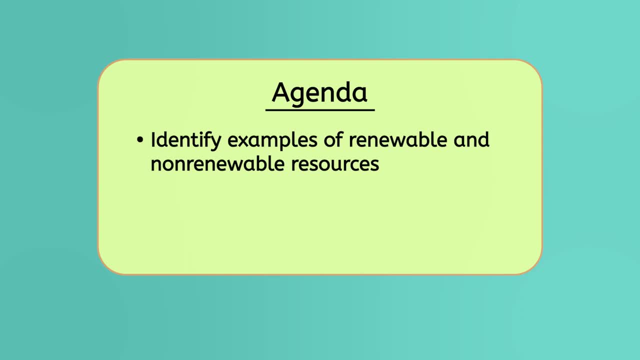 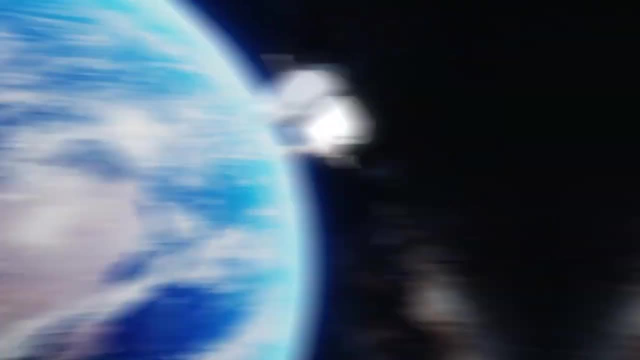 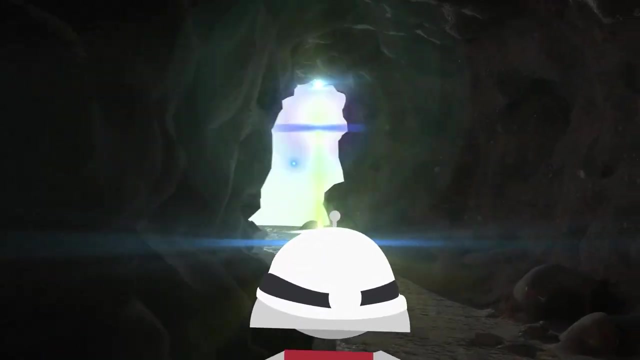 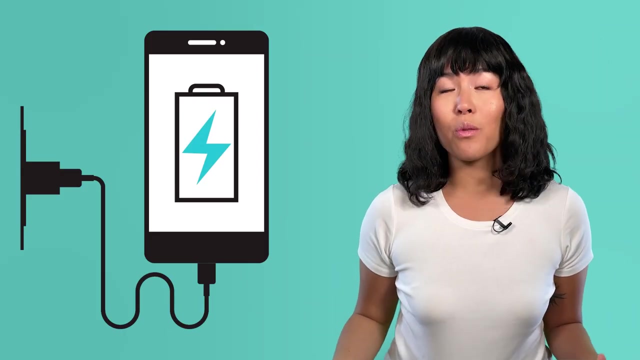 you'll be able to identify examples of renewable and non-renewable resources and explain what makes a resource either renewable or non-renewable. Let's get started INTRO. Whether we're charging our phones or drinking a glass of water, we're all constantly using 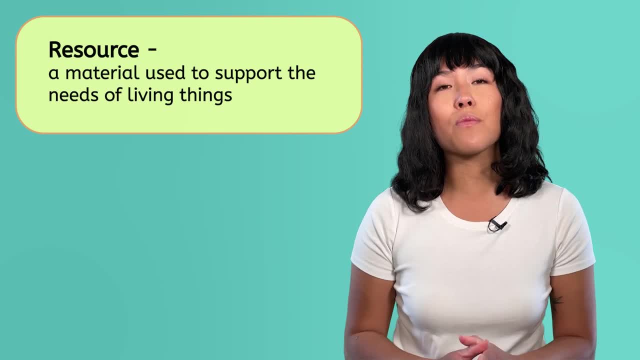 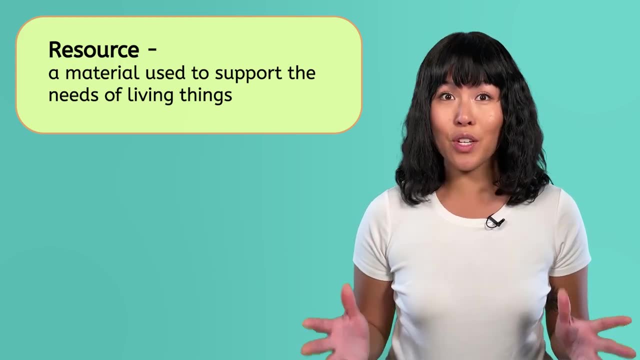 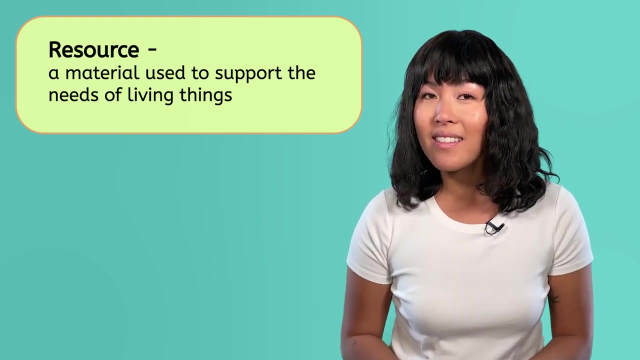 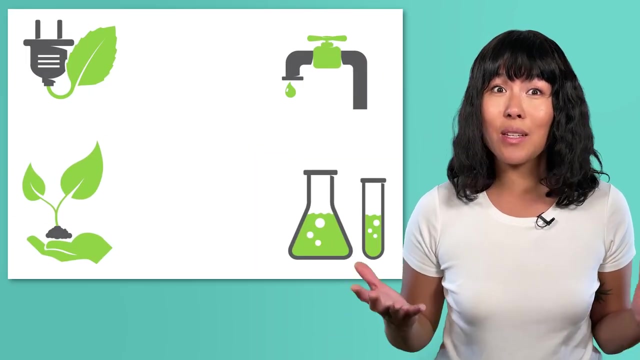 resources. A resource is a material used to support the needs of living things like the need for food or shelter. Humans are constantly using resources to generate energy, grow food, manufacture goods, build houses, create medicine and more. So how do we make sure we have enough resources for all 8 billion people on Earth? 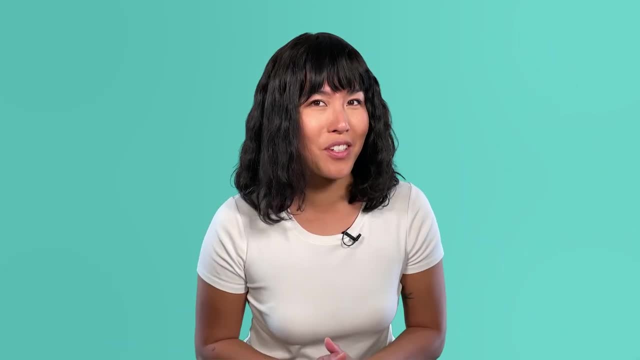 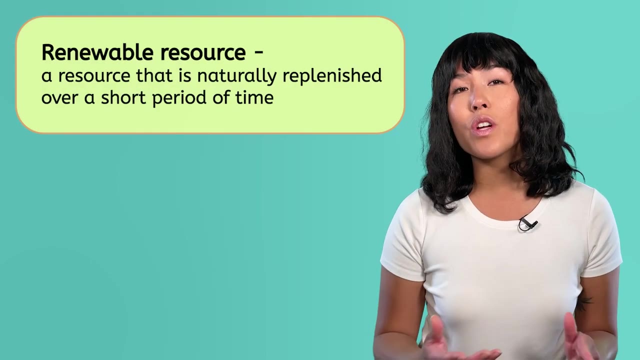 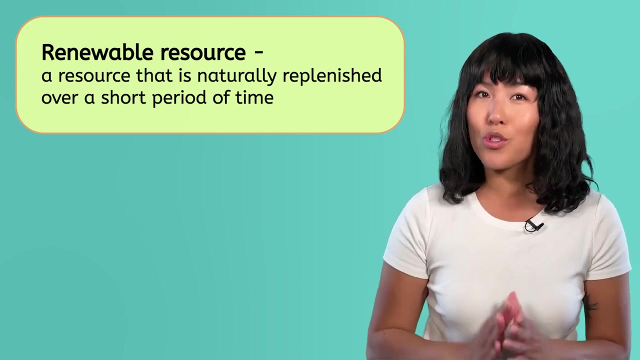 Won't we run out at some point? Well, I have good news. There are some resources that, no, we really won't run out of. We call these renewable resources. A renewable resource is a resource that is naturally replenished over a short period of time. In other words, it's a 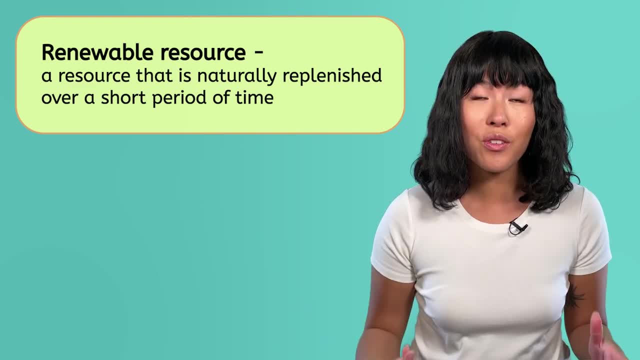 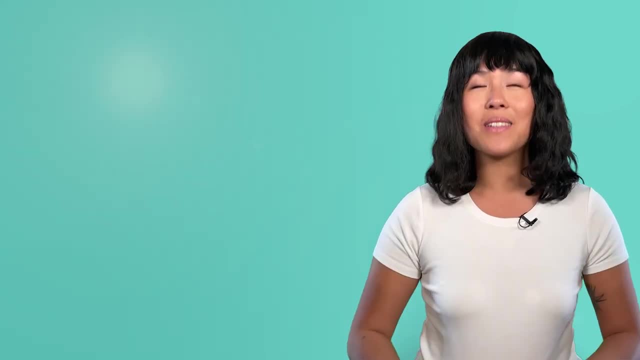 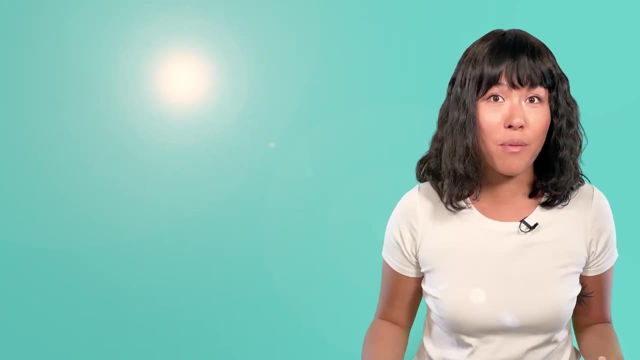 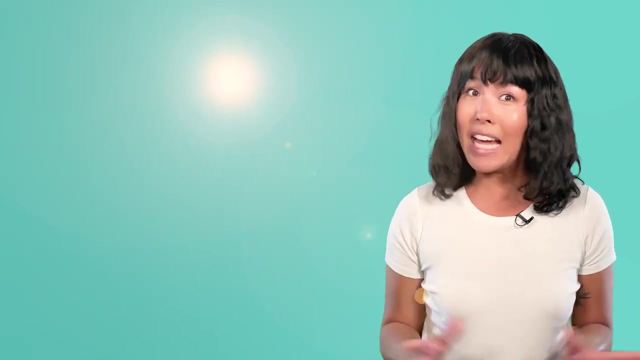 resource that we're not likely to run out of because it's replaced faster than we can use it. A great example of a renewable resource is… SUNLIGHT. In just one hour, our planet receives more energy from the sun than everyone on Earth uses in an entire year, And the sun isn't going to run out of light anytime. 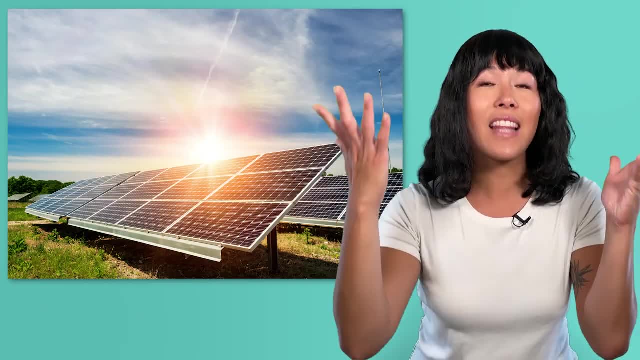 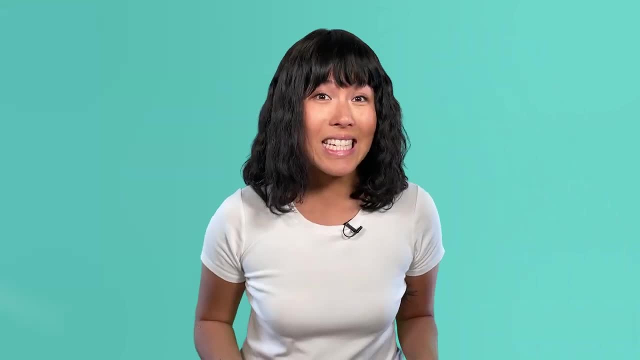 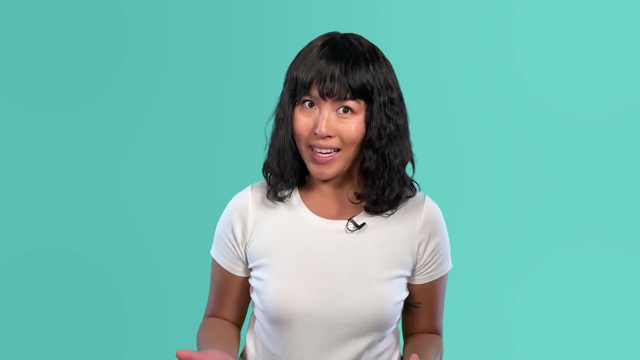 soon. We can use our endless supply of sunlight to generate energy, Which is why solar panels are becoming more and more common. Wind is another renewable resource. As long as the sun is causing global patterns of heating and cooling, we'll have plenty of wind. People have used this renewable resource. 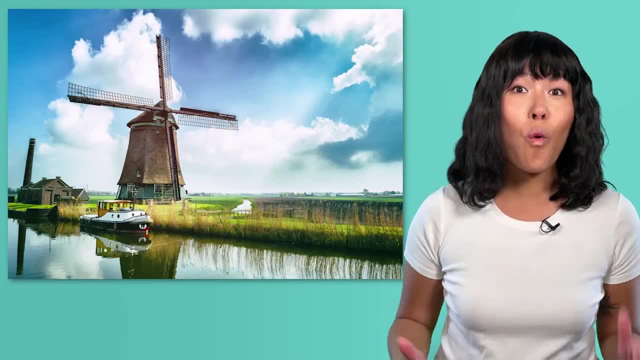 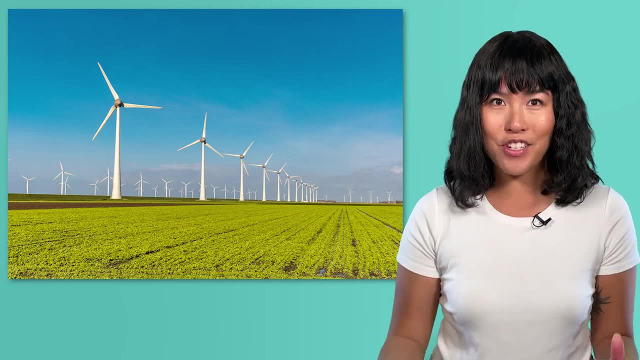 for centuries to push sailboats and turn windmills. Nowadays we use wind turbines to harness the force of wind and turn it into energy. This is why solar panels are becoming more and more common. They're used to push windmills and turn windmills. Nowadays we use wind turbines to harness the force of wind and turn it into energy. 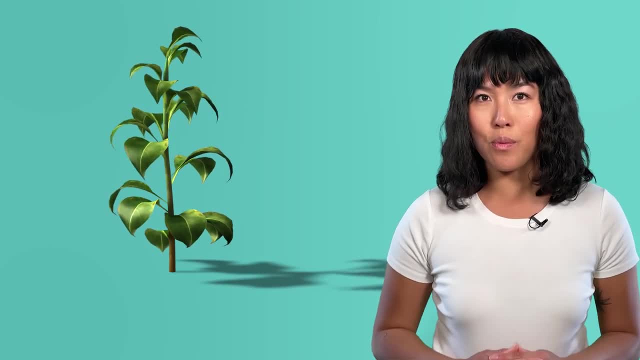 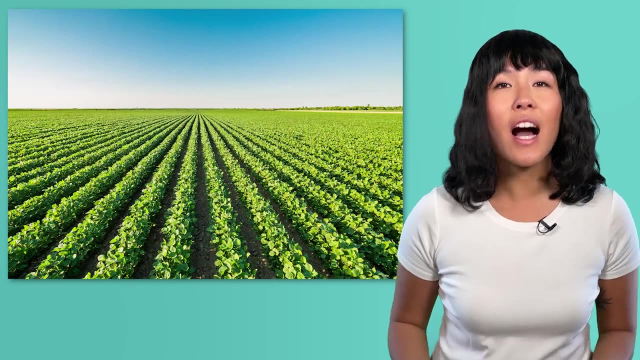 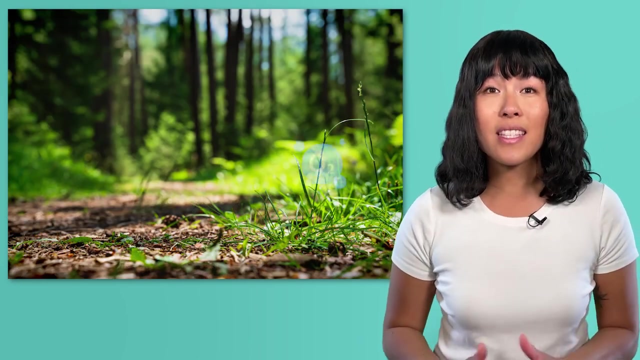 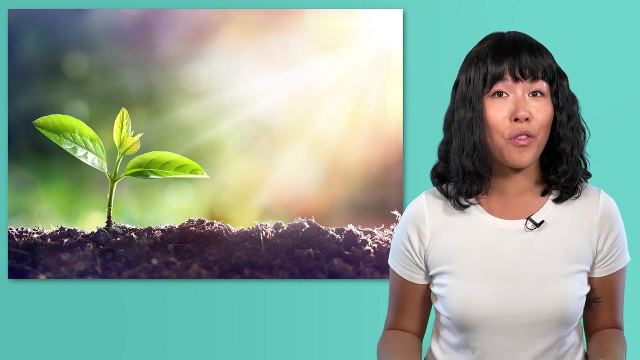 Plants are another important renewable resource. We use the wood from trees for building houses and making paper, and grow tons of different plants for food. Even the plants that we don't directly use are still helpful, since they produce the oxygen we breathe. New plants grow and naturally replace the ones we use over time, and we often help this. process along by farming too. However, trees and plants can become non-renewable if we harvest them faster than they're able to grow back. We have pretty stable access to renewable resources like sunlight, wind and plants. However, non-renewable resources take an extremely long time to replenish. 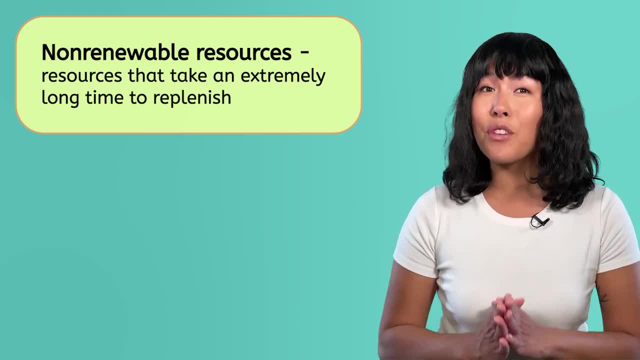 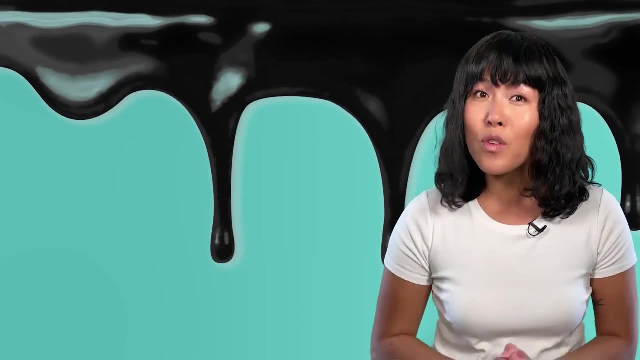 They're used up much faster than they're replaced, meaning it's very possible we'll run out eventually. Fossil fuels like oil and coal are some of the most important resources we have Some of the non-renewable resources we use the most. 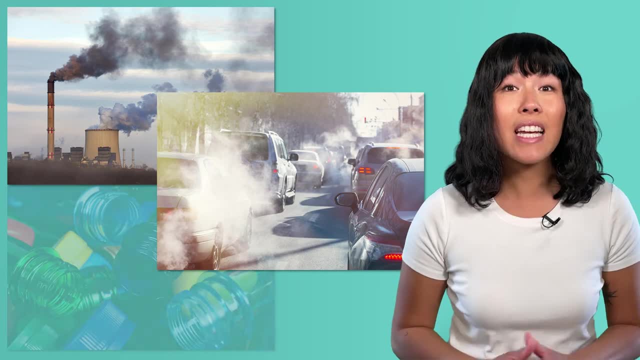 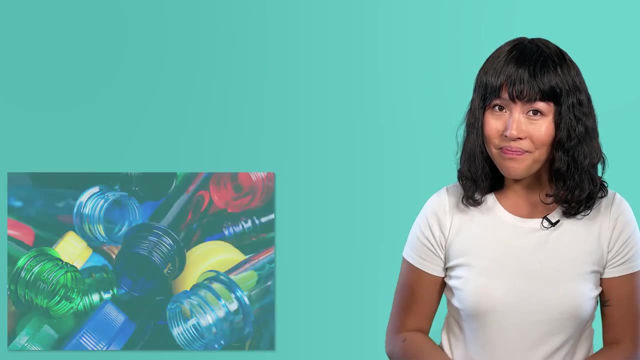 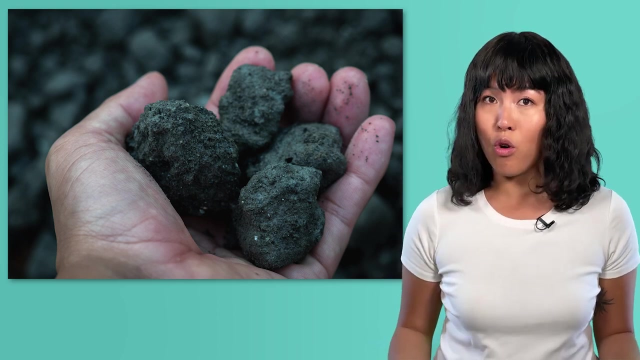 These fuels are used to generate electricity, to power cars and even to make plastic. Most people use these resources every single day. However, our planet won't be getting more fossil fuels anytime soon. They take millions of years to form and we use a lot of them. 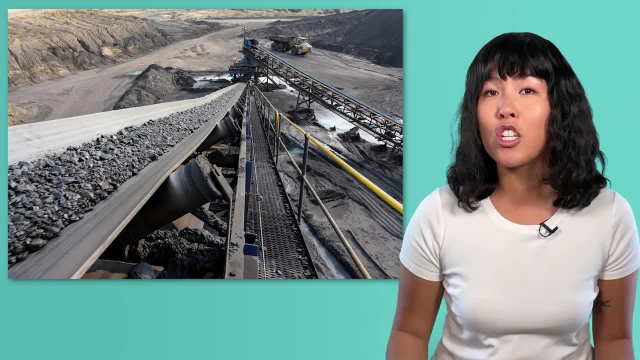 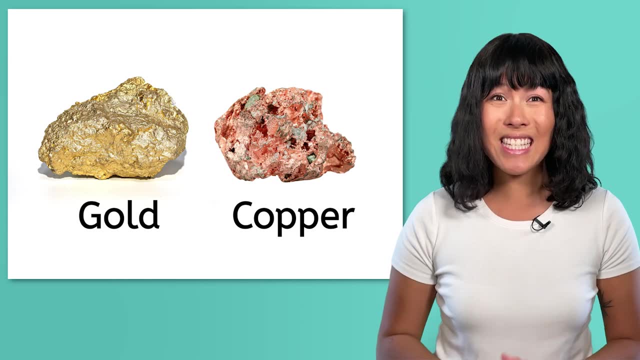 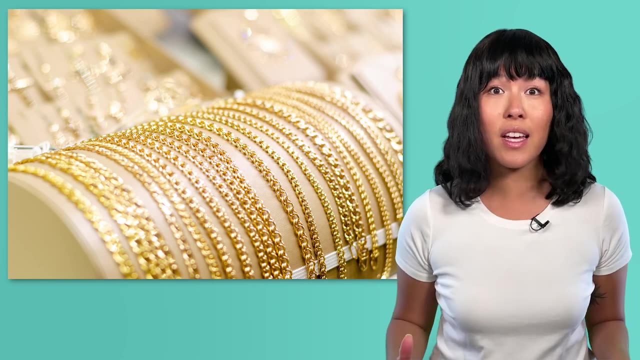 We're on track to run out of fossil fuels in under 200 years, But these fuels, like gold and copper, are also non-renewable resources because it takes such a long time for them to be replenished by the rock cycle. We use these metals for all sorts of things, from jewelry to the conductors in our cell. 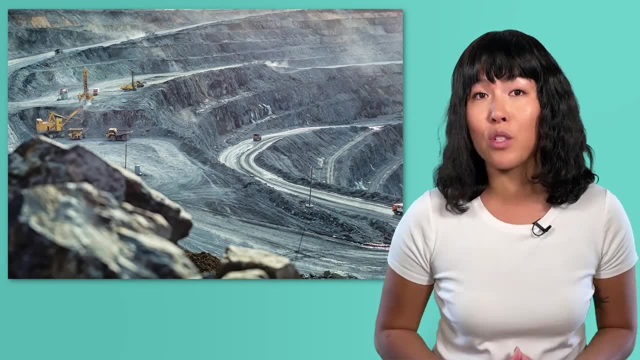 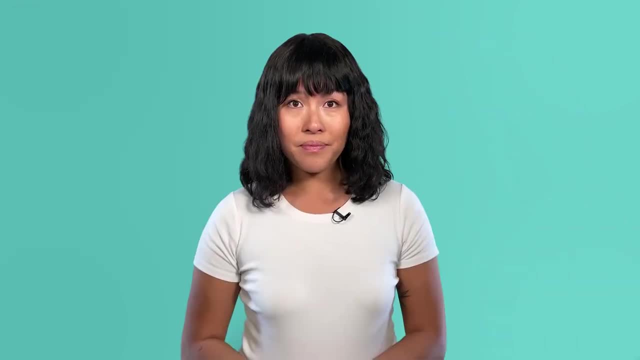 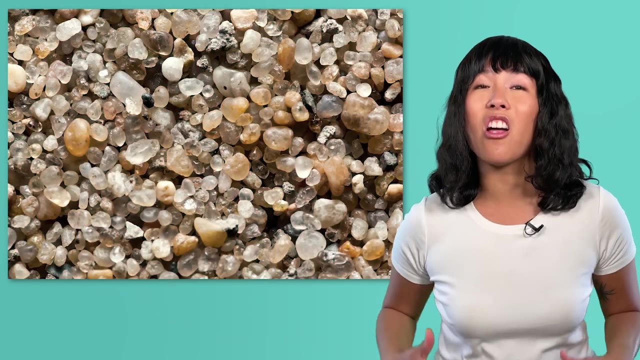 phones. We mine thousands of pounds of both of these resources every year, and at this rate we'll run out of them before long too. This one might sound surprising, but sand is also a non-renewable resource. Sand takes a long time to form, since it's made of rocks and minerals that are broken. 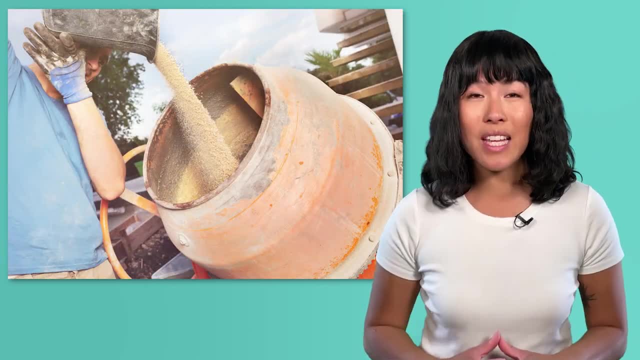 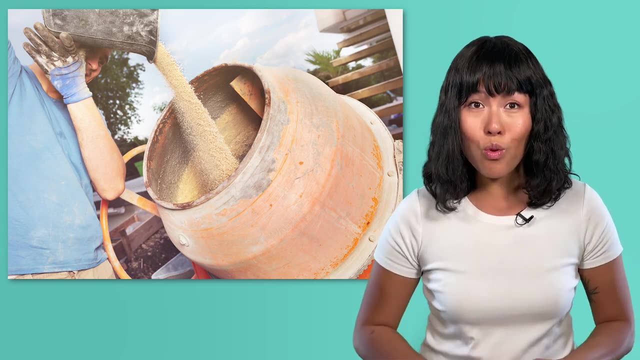 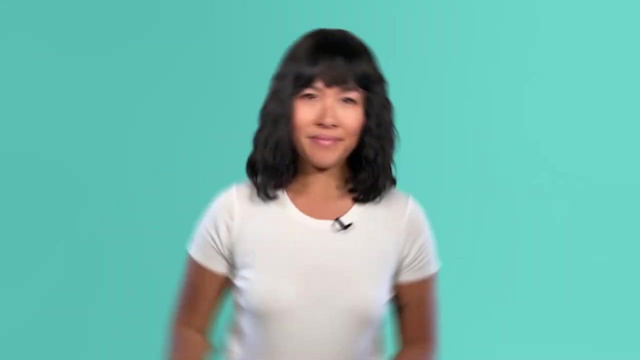 apart. during the rock cycle, We use tons of sand in construction jobs to make materials like concrete. In fact, it's the second most used resource on our planet, and we're using it up much faster than the rock cycle can replace it. Most resources on our planet are either renewable or non-renewable. 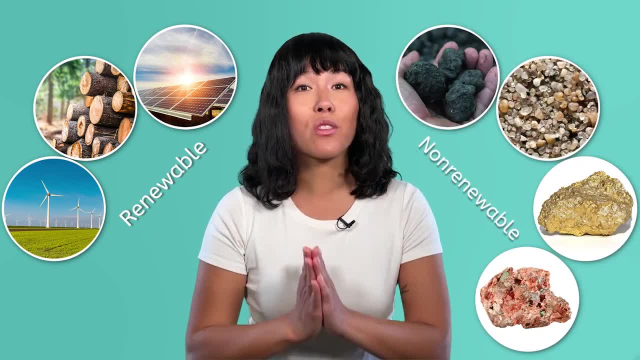 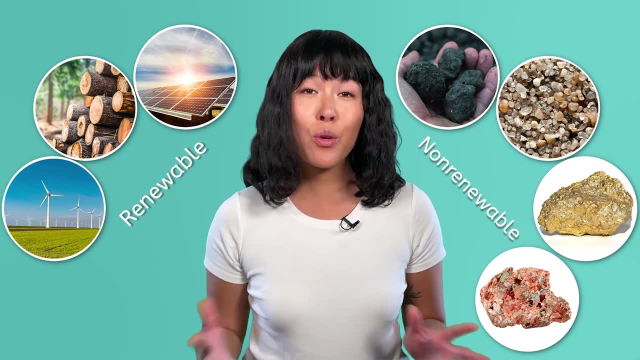 So what are these resources? Well, there are several, depending on how long it takes our supply to replenish. However, there are a few that Earth scientists can't quite agree on. Two of the resources in this in-between category are water and soil. 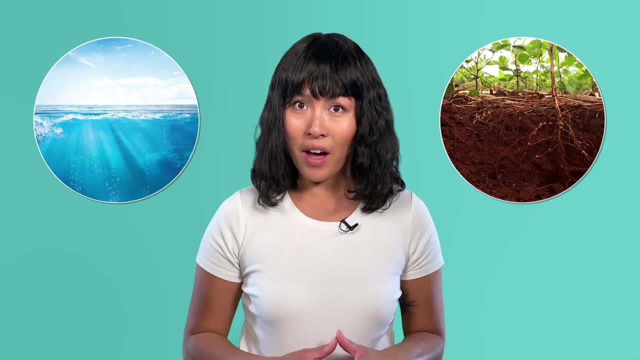 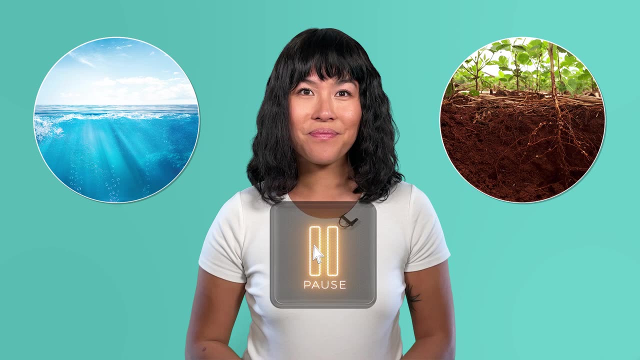 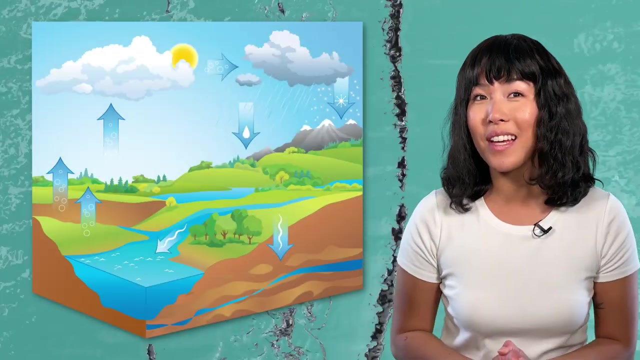 Why do you think these resources are so hard to classify? Pause the video here and record your thinking in your guided notes. Let's look at a resource we all use every day: Water. Thanks to the water cycle, this precious resource is constantly replenished as it moves through. 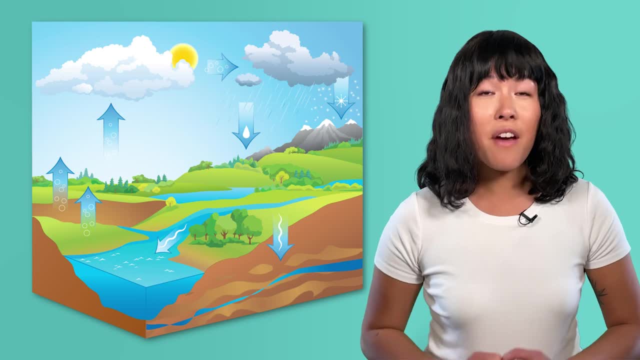 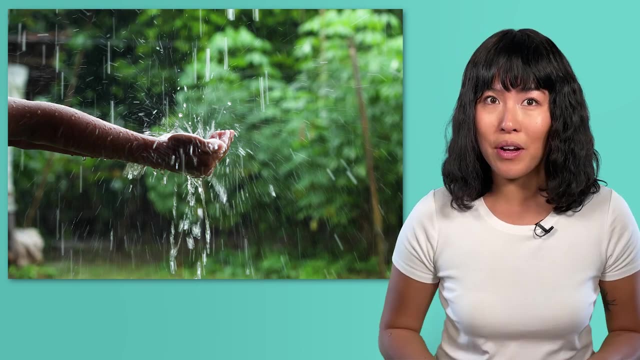 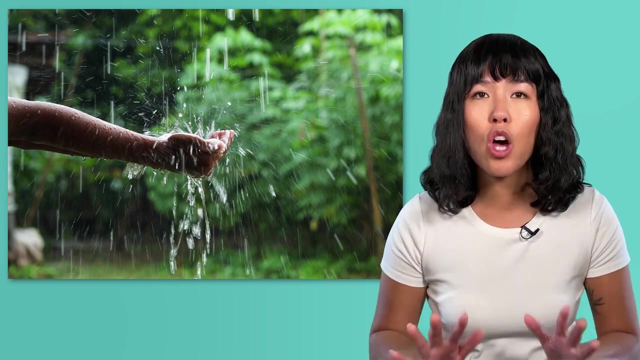 the Earth's system. But, as you might remember, very little of the water on Earth is usable freshwater. While the water cycle does replenish this small amount of freshwater, we use water faster than it's being replaced. That's why water conservation is so important. 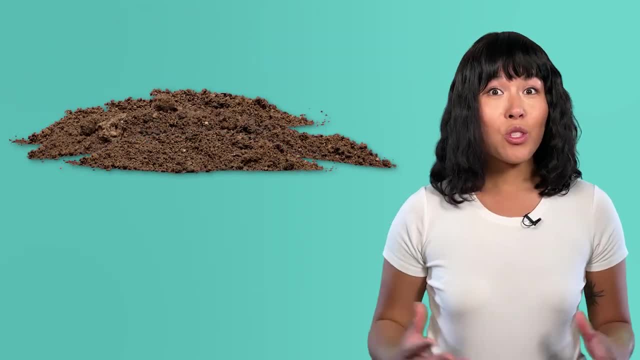 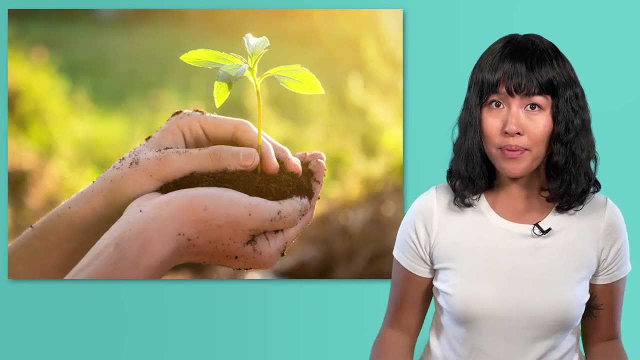 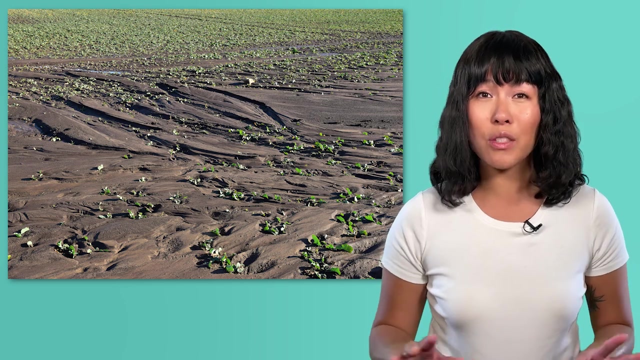 We definitely don't want to run out Soil. It's even harder to categorize than water. If we carefully manage how we use soil when growing crops, it can be replaced faster than we use it, making it renewable. But these careful practices aren't always followed and soil forms extremely slowly. 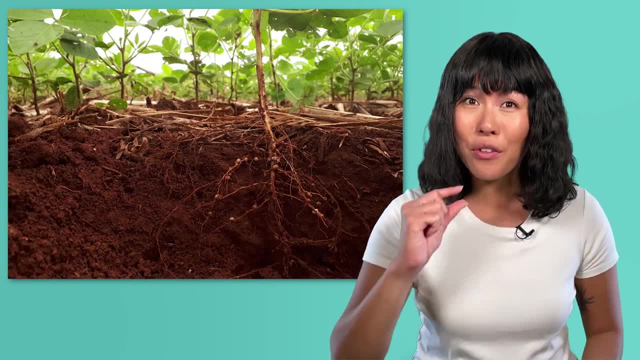 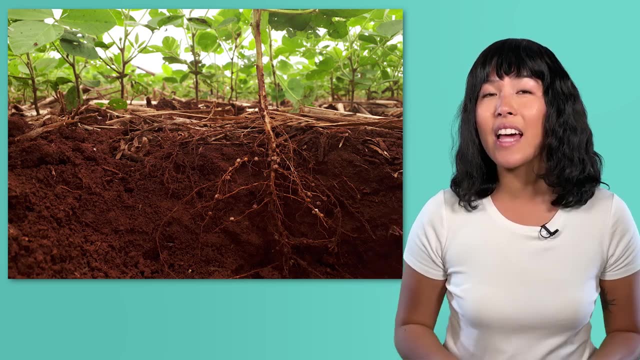 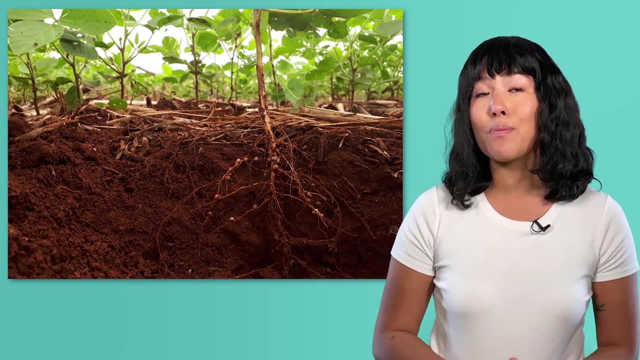 It can take over 500 years for a single inch of soil to form, making it easy to see how it can be considered non-renewable too. It's status as a renewable or non-renewable. Well, it depends on where the soil is and whether or not it's being cared for. 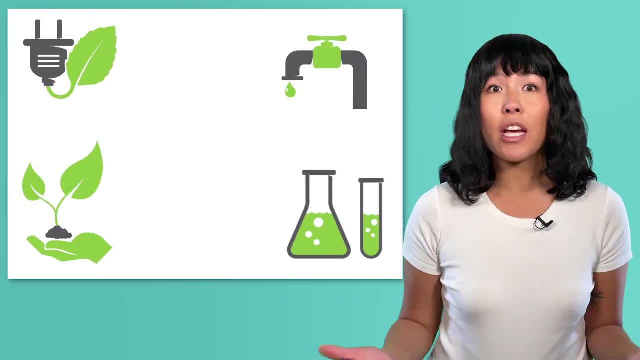 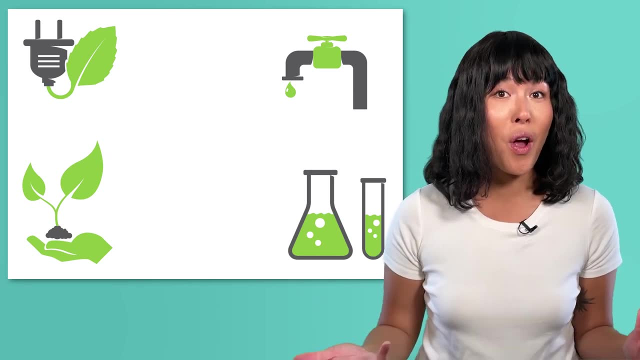 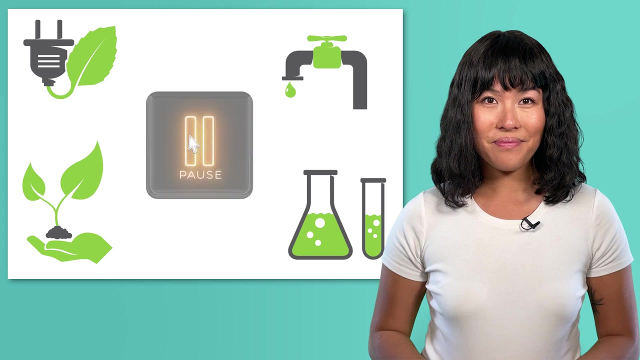 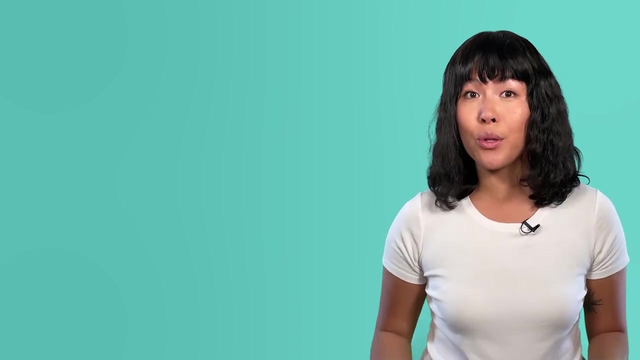 So what do you think the solution is? What should we do to make sure we have enough resources for everyone on Earth, especially as our population continues to grow? Pause the video here and record your thoughts in your guided notes. Most Earth scientists think that one of the most important things we can do to ensure 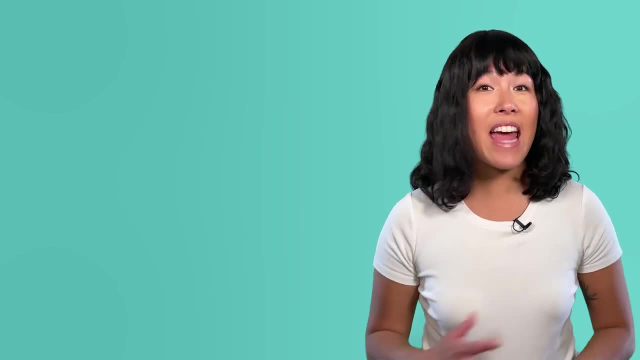 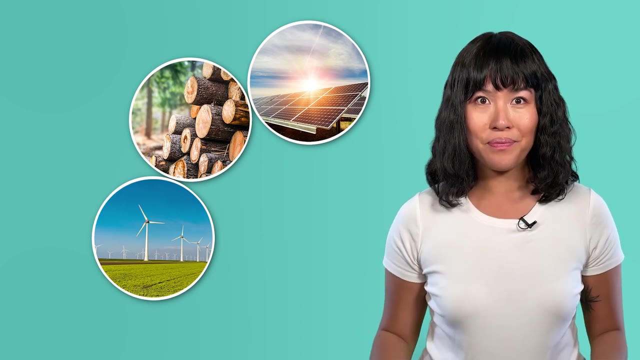 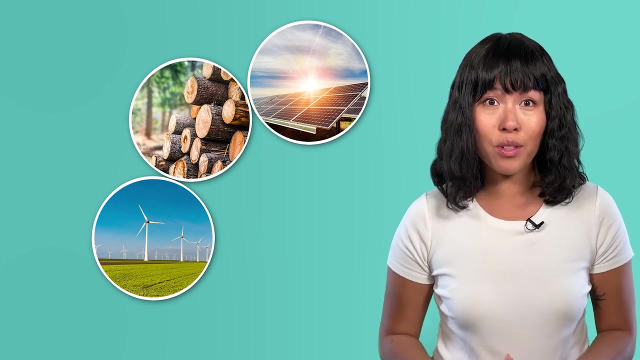 we have plenty of food, energy, medicine, and everything else we need is to try to use renewable resources whenever possible. In our next lesson we'll take a closer look at the steps we can take to carefully manage our planet's resources and what can happen if we don't.